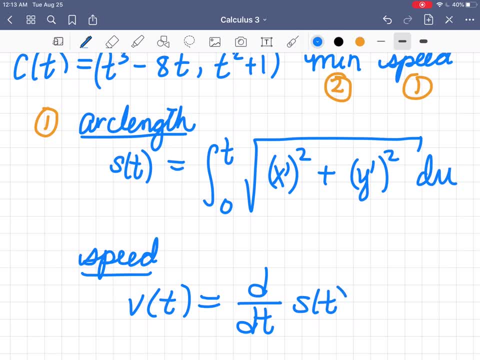 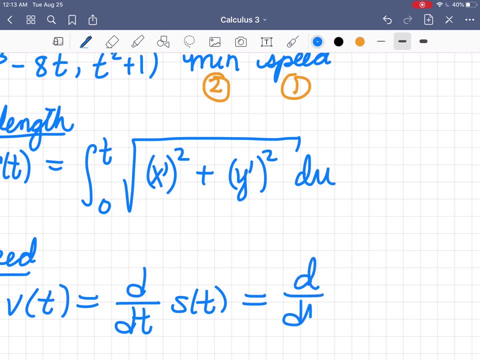 length. Okay, so what we're doing ultimately is we're taking the derivative of this integral, and the fundamental theorem of calculus says they undo each other, right? So these two things basically undo each other. all right, Let me go ahead and I'm gonna copy all this here. 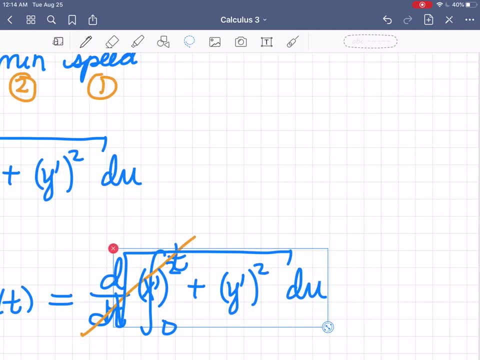 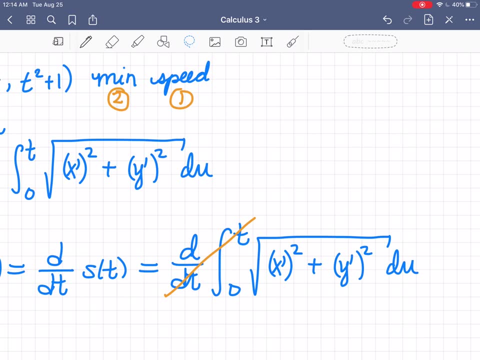 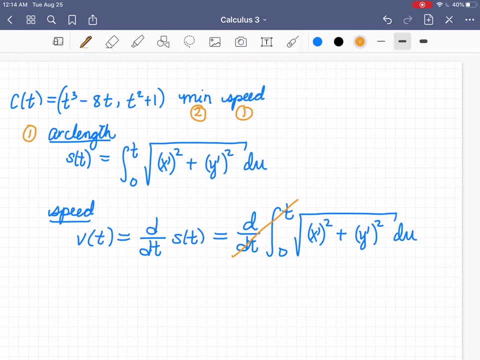 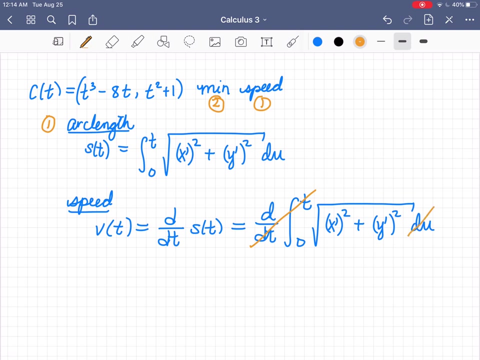 All righty, Scooch it over, All right. So what I'm saying is: a lot of things get taken care of here when we're computing the speed, because when you're taking the derivative- derivative of the integral- you don't actually have to integrate. okay, you end up getting just 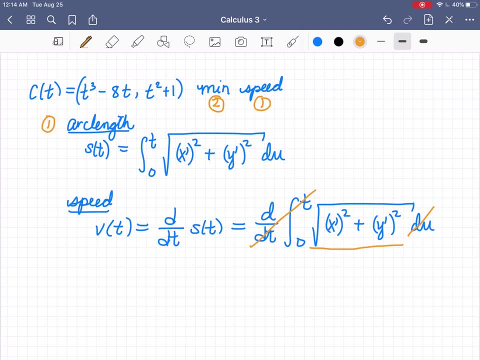 the integrand with the t plugged in. okay, so the speed ends up being square root, x prime squared plus y prime squared. okay, so in our particular problem, here's our x and here's our y. we're going to go ahead and plug those in, taking derivatives, squaring and all that. 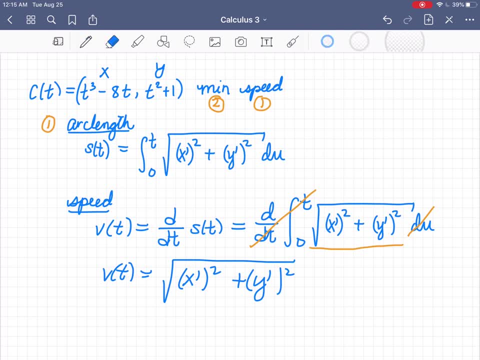 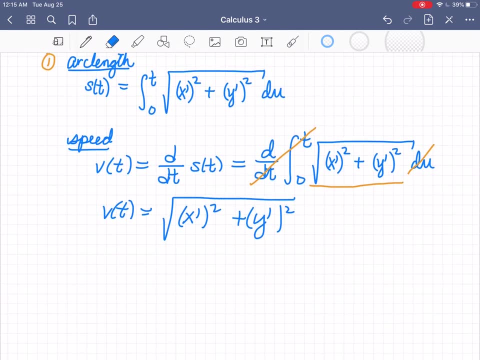 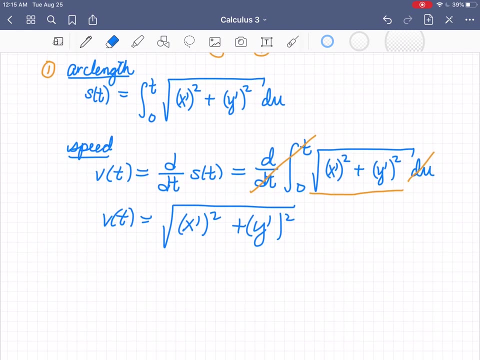 so when you do this- and let me go ahead and scooch that up if I can, okay, so x is 2 t cubed minus 8 t, so its derivative is 3 t squared- I think I need to move this. I think I need to move this. 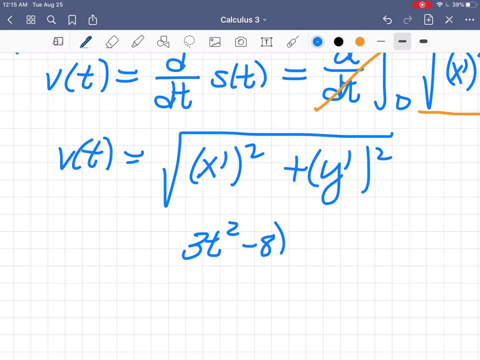 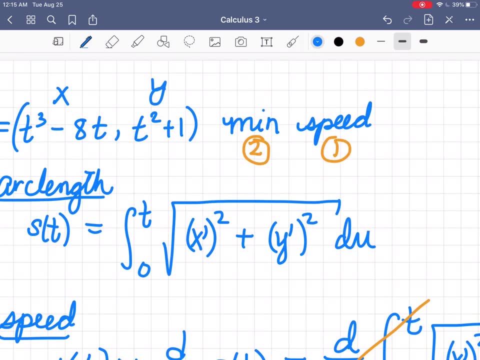 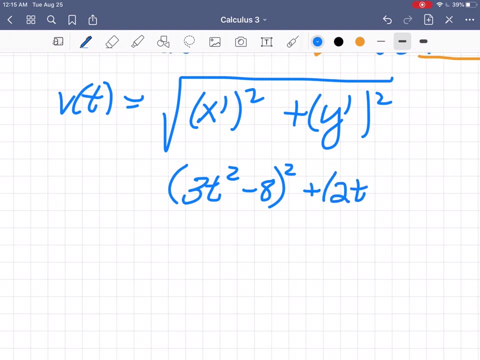 bigger a little bit minus 8. okay, so that's x prime. y prime is scooch that t squared plus 1. so we end up getting 2 t for y prime. that needs to be squared, all right. so this is V of T for our particular function and 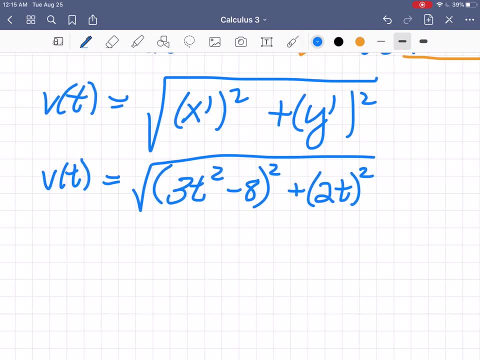 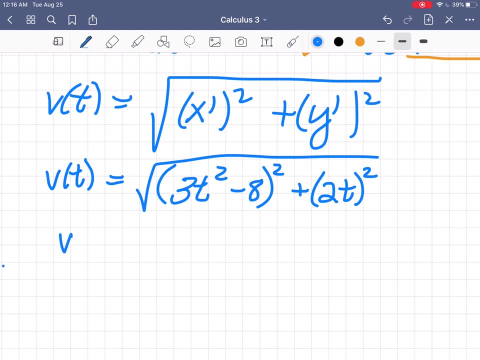 I think the book says: why don't you go ahead, square the speed and take the minimum of that function? so the square of the speed would end up being just 3 t squared minus 8, all of that squared plus 4t squared. and if you expand this piece, 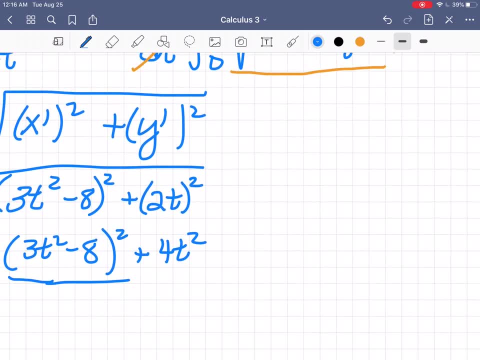 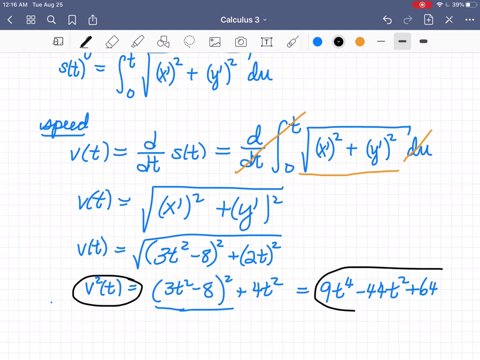 right. here you end up with, okay, 9t to the fourth, and then minus 24 times 2 is 48. so minus 44, minus 44, that's right. t squared plus 64. so this- let me scooch that out- is v squared, the, the speed squared. and we're going to go ahead and now minimize. 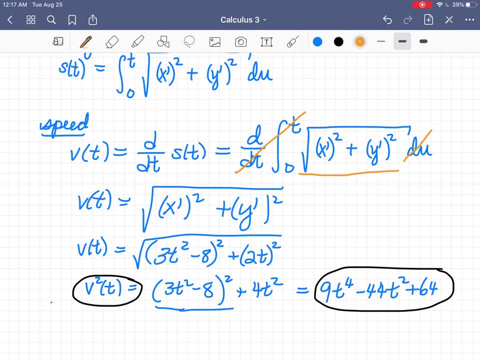 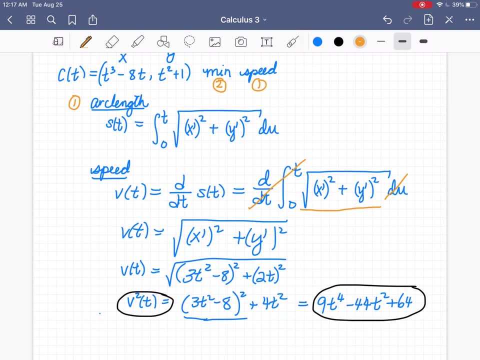 this function right here. okay, so part two. okay, so this is part one. is we've got this function. we computed this is the speed excuse. this is the speed function. well, the speed squared, but this is the function right and the the hint was: we want to, we want to minimize this now. 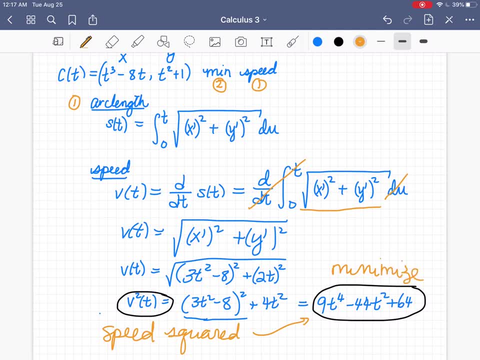 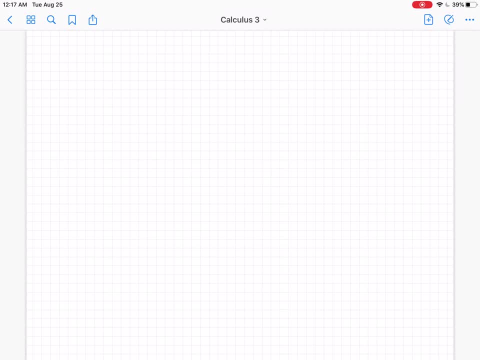 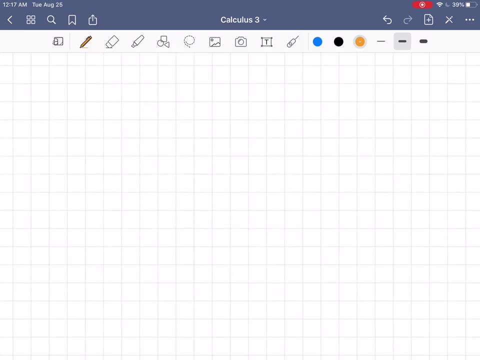 i'm going to go to the next page and do that, all right, so now this is part two: minimizing. okay, okie, dokie, uh, we want to minimize what i said was v squared, and then we're going to go to the next page and do that. all right, so now this is. 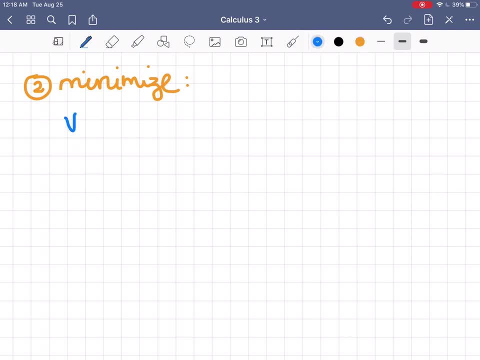 v squared. v squared, which is 9t to the fourth minus 44t squared plus 64. how do we minimize? well, we got to go back to calc 1 and remember that what we got to do is take a derivative, and then we're going to go to the next page and do that. all right. so now this is part two: minimizing. 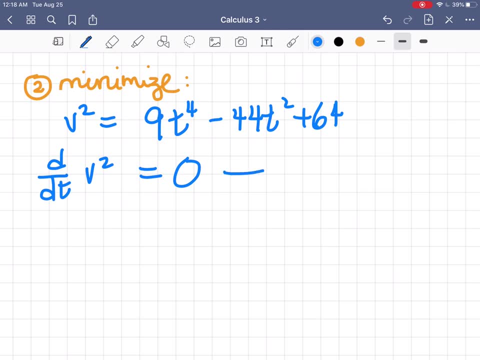 all right, so we're going to go to the next. set it equal to zero, and then you get these critical points, and then those critical points will tell you where you have max's and min's. okay, so if we compute the derivative of v squared, well, that's a simple.